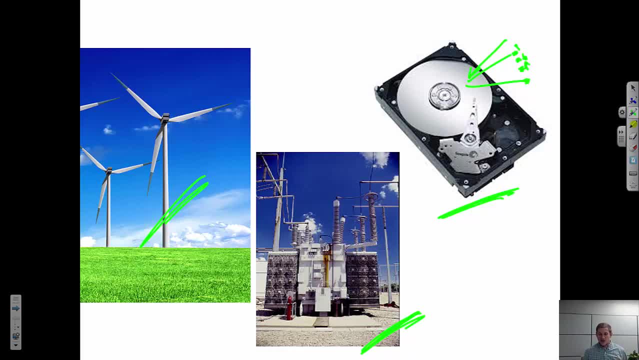 usually a soft ferromagnet, so typically something like iron that's wrapped a different number of times between one wire and another wire And this steps the voltage up or down. So in all of these cases we need to have magnets and magnetic materials that perform some specific tasks. They have to have some 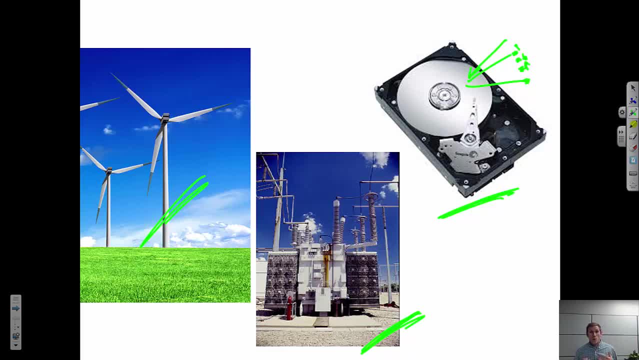 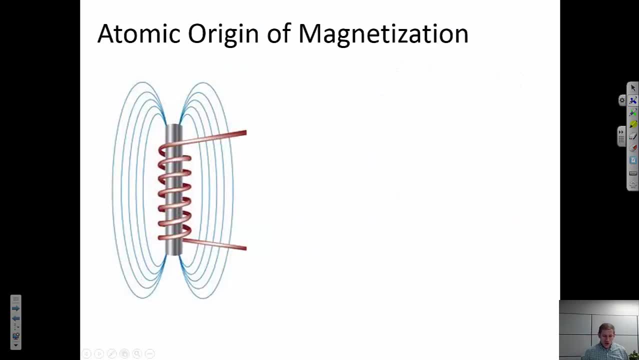 specific properties. The point of this video is to think about where does magnetism come from? in materials, And we're going to start off with the classical picture of taking a metal and we can wrap a wire around it, And when we do that, if we flow current through the wire, then we generate a. 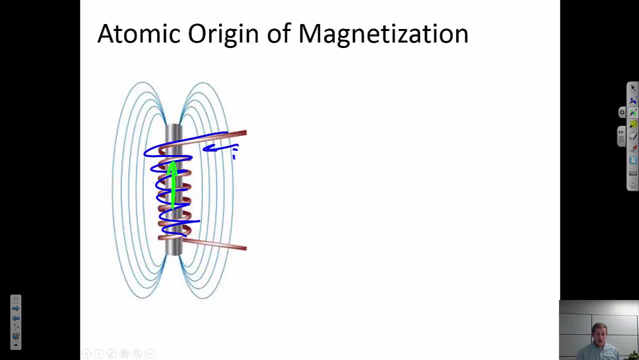 magnetic field. So we'll generate a strong magnetic field within that loop of wire. And if we have a soft ferromagnet in here, something like iron, it's going to get even stronger And you can see the stray field that comes out around, because all of the 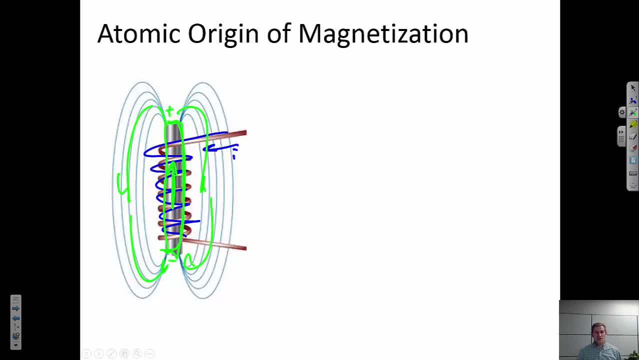 magnets that we're familiar with are dipoles. There's a positive and a negative side. There's no magnetic monopole that has been observed to exist. So from this picture we think of moving current as being required to create a magnetic field. So what about in a magnetic material? I don't think about there as 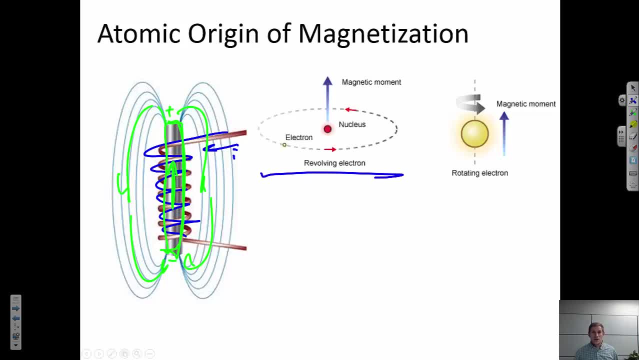 being moving current, but on the atomic level you can think about the electrons moving in the system right. So electrons within an orbital are always moving, and so there could be some sort of an orbital contribution to magnetic moment. Also, electrons themselves can have an inherent property that we typically call. 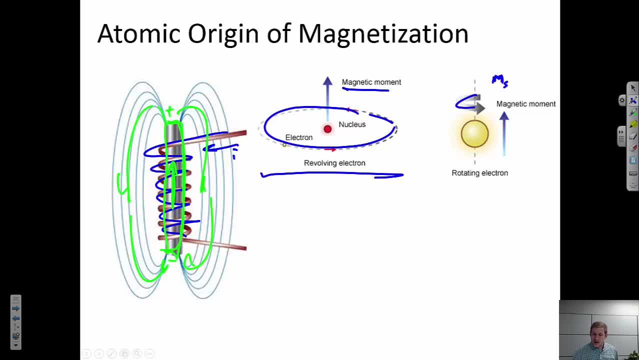 spin And that's given by the quantum number m sub s. And so the picture that some people like to draw is this electron spinning like a top. Again, we're sort of imposing our classical picture of things spinning on it. That's not necessarily the best physical picture, but we don't really have a good. 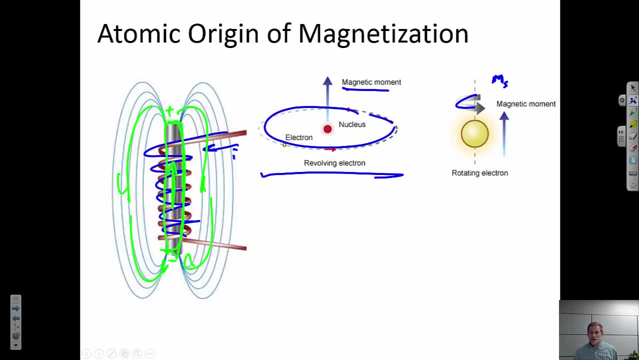 physical picture. So we just know that there's some inherent property of electrons themselves that leads to this magnetic moment from the electron contribution. So these two things interact And so in any atom, if I have unpaired electrons, I could have some magnetic moment contribution from either. 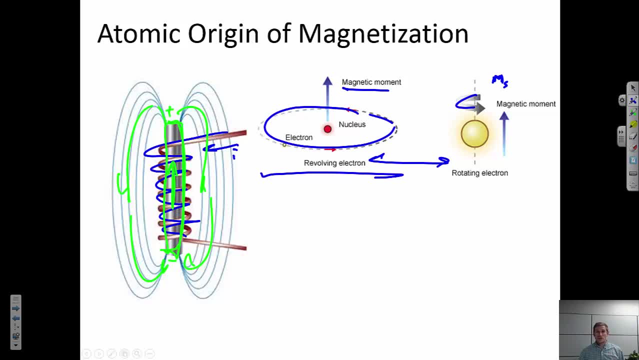 the spin or the orbital contribution or spin Or some kind of combination thereof. So the combinations get a little bit tricky and we're not really going to go into those here. This is based on quantum mechanics but you can understand the different potential magnetic contributions. 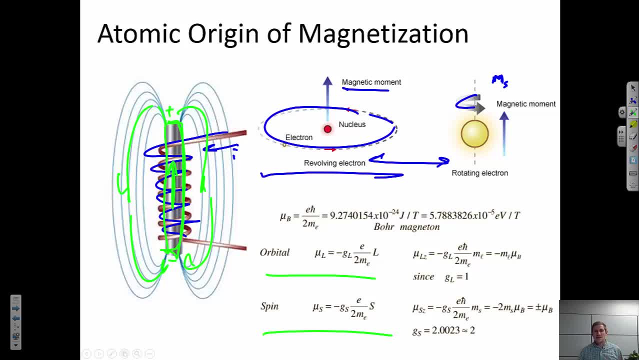 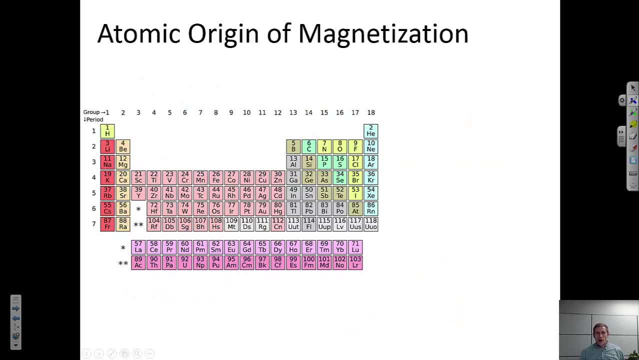 based on what quantum numbers are satisfied in certain elements. So let's look at a general periodic table Now. remember I told you that we need to have unpaired electrons to get this magnetic contribution, And so what that means is a couple things. First of all, the noble gases are never going to have a residual. 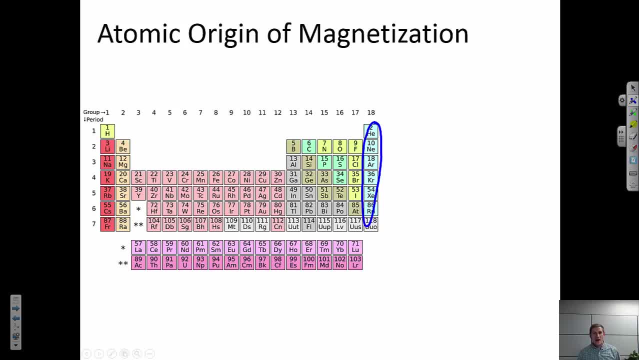 magnetic moment because they're always closed-shelled. You never have unpaired electrons, So the things that tend to be the most magnetic are those that are kind of in the middle of the transition metal series, because we can have a lot of unpaired electrons here. 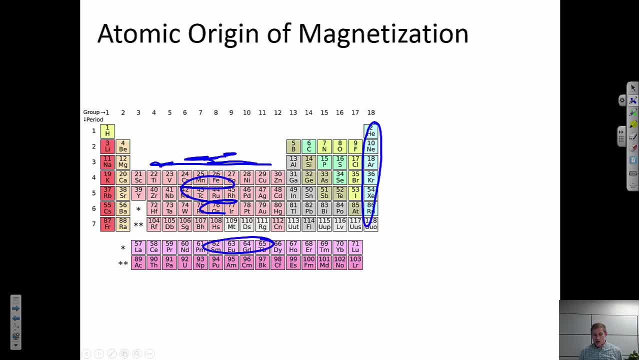 Or in the middle of the rare earth series, So we can have again. we can have a lot of unpaired electrons in the middle of these series, right? So think about, the rare earth has 14 electrons in those f orbitals, So I could have a maximum of. 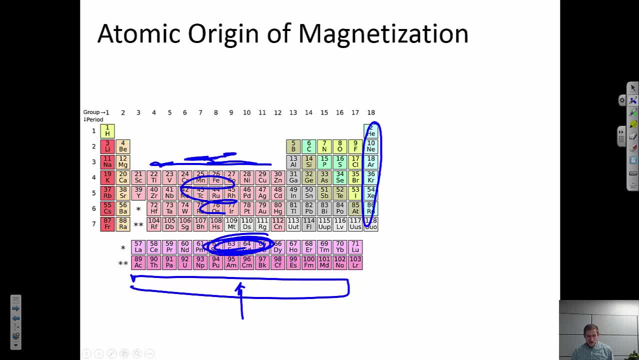 seven unpaired electrons in some particular state. So again, we're not going to go into what is the maximum moment that we could get for any particular atom. But the thing to remember here is that magnetic moments are particular to atoms And they're based on how many electrons are in those. 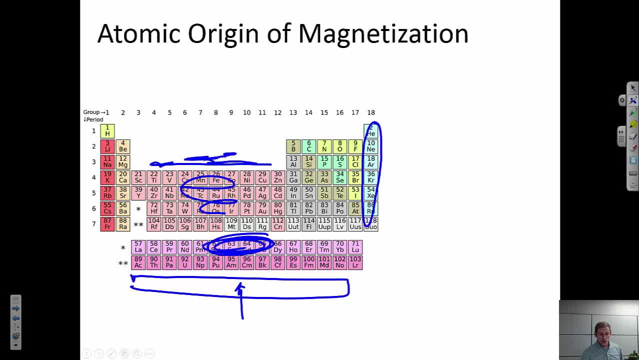 atoms and which orbitals are they filling. So, for example, iron would not necessarily have the same magnetic moment as iron 2 plus or as iron 3 plus, Because in each of those cases we have different numbers of electrons, and so orbitals are filled differently. 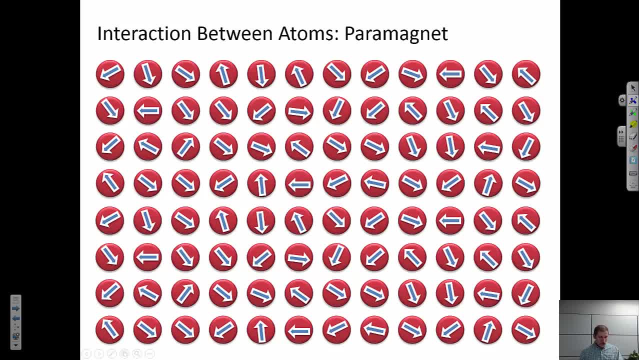 Okay, so we have this picture. Each atom can have some magnetic moment. A solid is just a whole bunch of atoms put together, right? So if each atom has an independent magnetic moment, so let's think about this one, and if it's not aligning with? 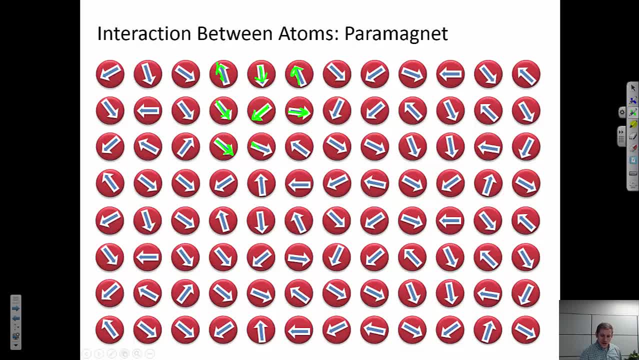 any of its neighbors, then I would get no net magnetization, So I would call this a magnetically disordered system. There is a magnetic moment on each atom, but they're not all aligned, so I would see no net magnetization in the system And we call this a paramagnet. Now, if I 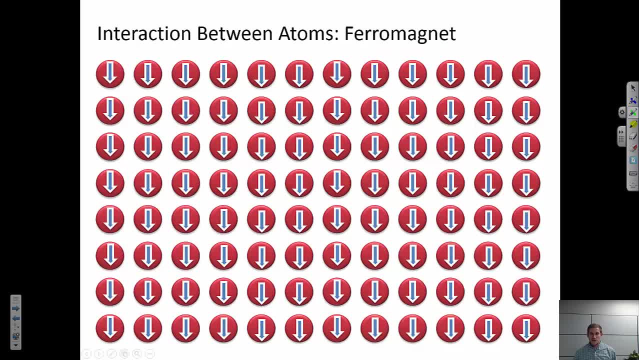 cool this paramagnet down. in some cases I can get all of those atomic moments to align, And that's what we call a ferromagnet. So this is what we think of as a permanent magnet, something that has a permanent magnet, A permanent aligned magnetic field, And in order to do that, it must have atoms that 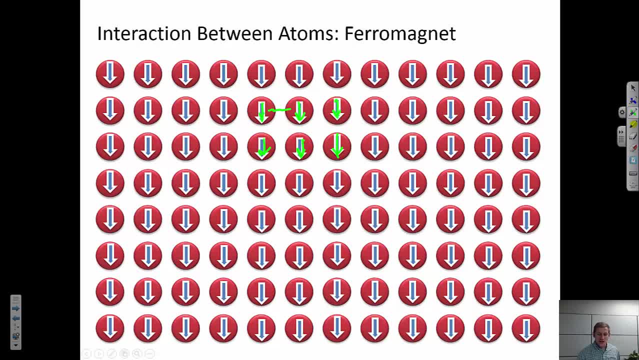 are aligned, There is some interaction energy between these different atoms. that says it's going to be beneficial. the whole system will establish a lower overall energy if they're all pointing in the same direction. So again, this is what we call a ferromagnet. Now, if I take any ferromagnet and I start heating it up at 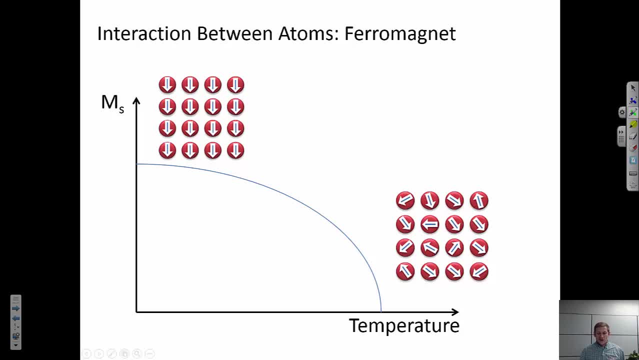 some point I'm going to put enough thermal energy in there that that thermal energy will overweigh the benefit I get from the atoms. the magnetic moments on the atoms lining up, So I would see a curve that looks something like this: The saturation magnetization, so the total magnetic moment that I could get in that 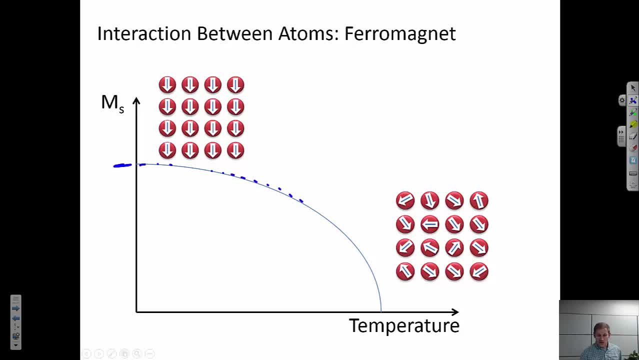 material will decrease as I increase the temperature, So I'm putting in more thermal energy. the system is becoming more and more disordered and at some point- and I would call this the Curie temperature- the system is no longer ordered. All of those atomic moments are now going to be free to take different 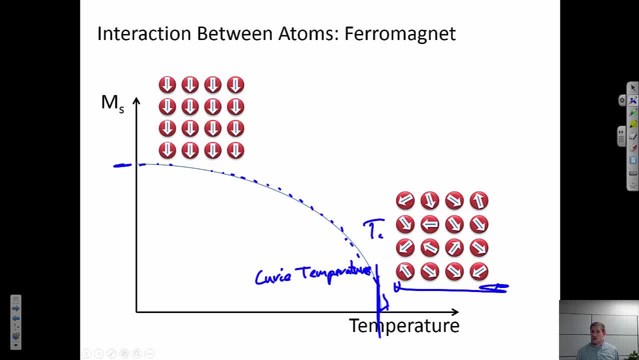 directions. So this is one kind of a transition in magnetic material systems, A transition between a ferromagnet and a paramagnet. All ferromagnets at some point, if I heat them up to high enough temperature, they'll become paramagnetic. So that's why I don't know if anybody would.